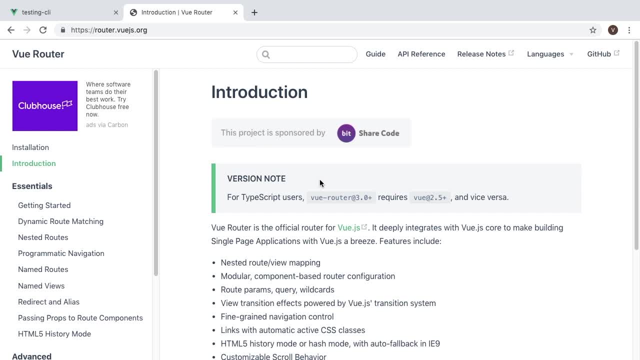 And they're a little bit harder to set up. But once you're set up, honestly it is no different than developing a regular website. So view router is the official router for Vue JS, So today we're going to be taking a look at how to get it installed in a project. 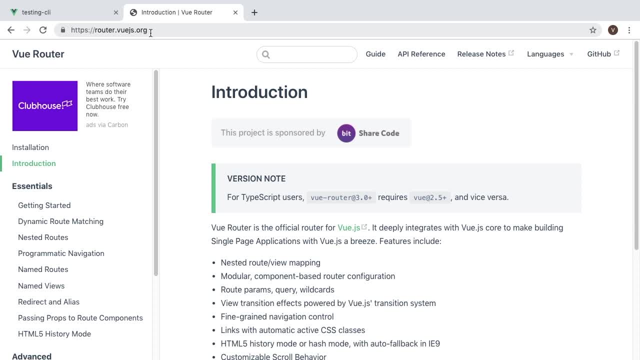 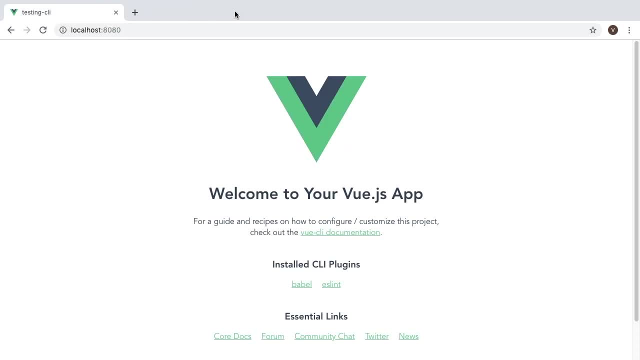 So the official documentation is under routervuejsorg, So definitely reference this documentation for any additional questions or features you'd like to discover. So I'm going to close this for now, And what I have here is just a simple view CLI application. It is a completely fresh. 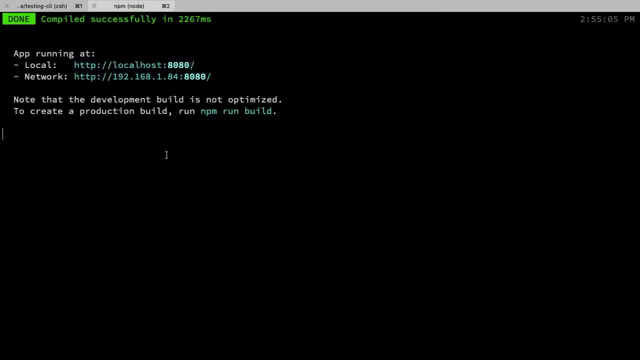 application. I haven't done anything for it. All I've done is just run the serve command. So in a new tab we need to pull in Vue router And we do that by running npm: install Vue dash router. this will pull in the Vue router package and plugin into our application. So now that 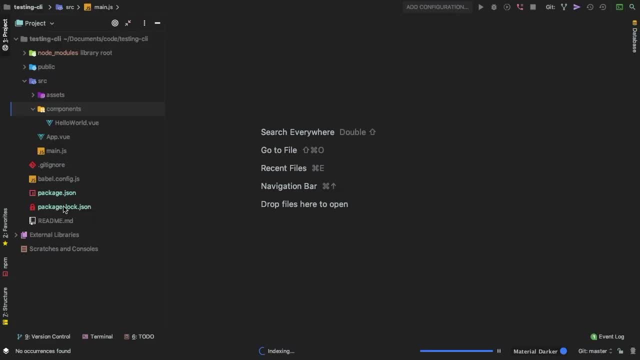 we have that installed, let's go ahead and start using it. So in my application here, we're going to start with the mainjs file. The very first thing you have to do is- and if you're not familiar with this, is the way that Vue defines plugins. Vue router is a plugin for Vue. 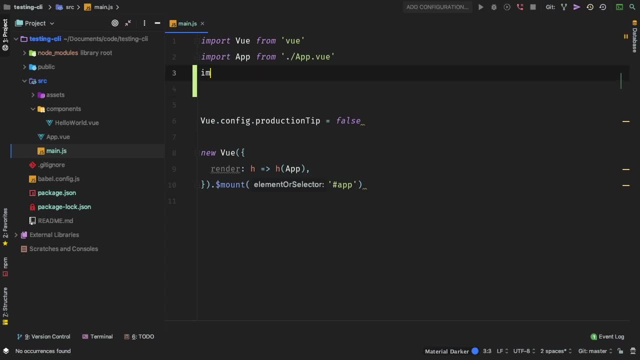 So, to use a plugin, what you have to do is, first and foremost, let's import Vue router from, and it's going to be just vu router, view dash router. So now that we have that imported, now we need to use it, And that's the key word that we're going to use. we're. 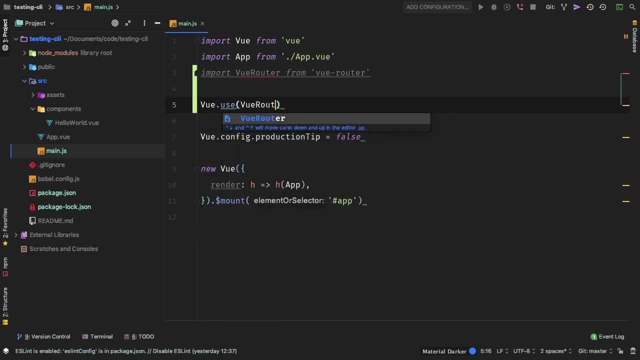 going to say view dot, use And let's go ahead and use Vue router. So this is basically telling view that this is a plugin that we want to use alongside with our Vue system, alongside with our view that we are importing up here at the top. So the next thing we need: 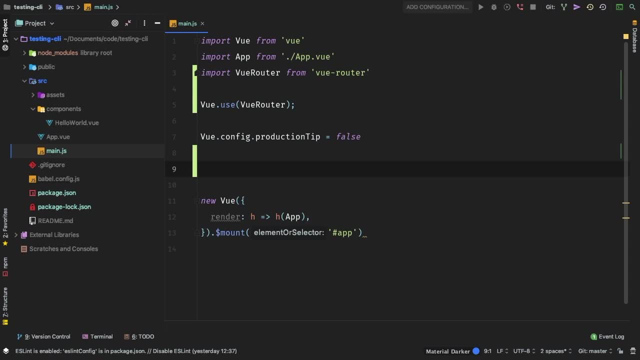 to do is define some routes. Now, if you watch the previous episode, where we basically created a router from scratch, the next thing you know we need is routes. So let's go ahead and create some routes, And we can do it in several different ways We can actually do. 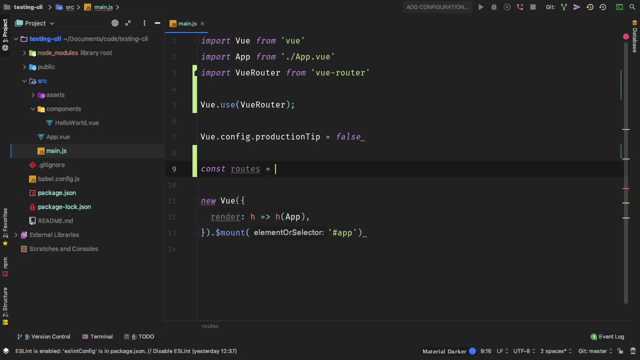 it like so, where we have routes that equal an array of routes, But I like the notation where everything is a little bit more compact. So what we could do is actually initiate a new view router and inside of that then declare our routes. So why don't we take that approach? 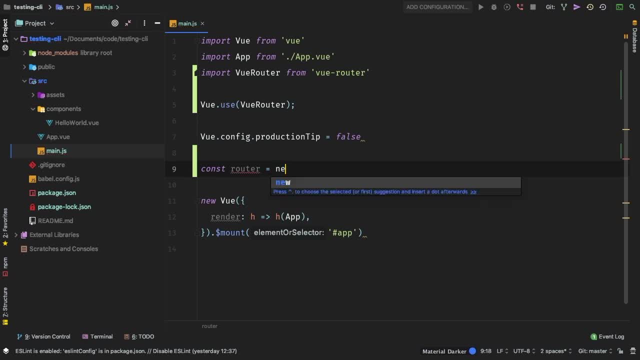 So we're going to say const router And this is going to be equal to a new view router, right? So we need to make an instance of view router So we can start defining our routes. Now this is going to accept an array And inside this array, the first key we're going 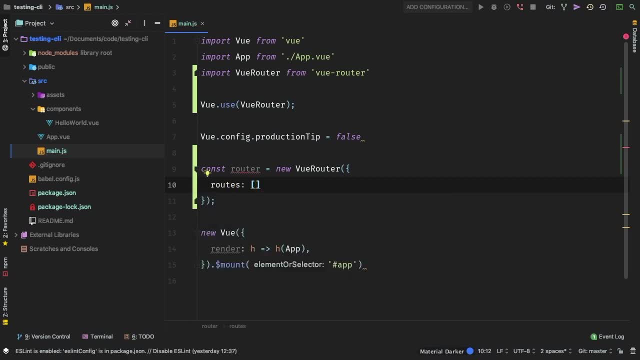 to pass in is route. And again, this is no different than just declaring your route in a separate view, variable, But this just saves you a little bit of lines, But either way it would work. So inside of here, every route is going to need two parameters. The first one is going: 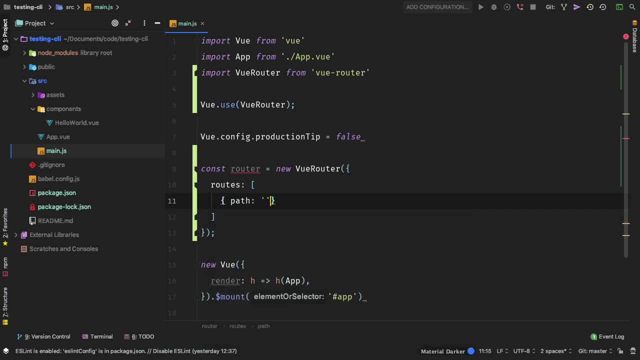 to be path, And that's going to be equal to some sort of path, meaning a URL that you want to visit, And the second one is going to be a component, meaning the component that we're going to load. So why don't we load? Hello world, this is a component that just comes. 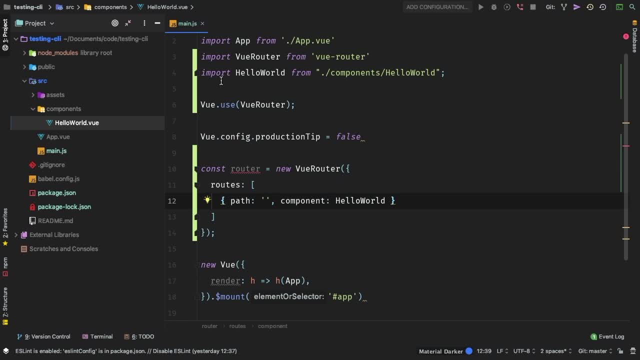 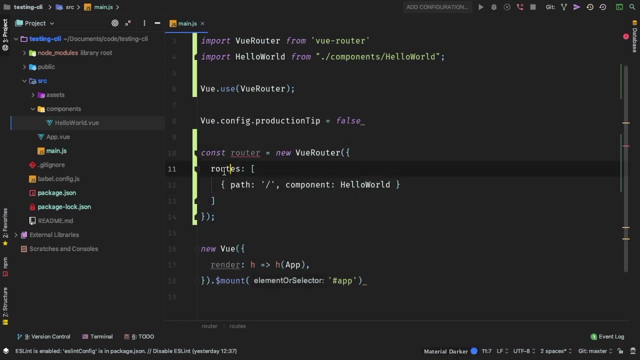 pre installed with any view CLI application And if you notice up here at the top, it did get imported For me automatically, just a feature of my ID. So the path that we're going to add is just a slash, meaning just your regular home page. So now we've got our router, we've got 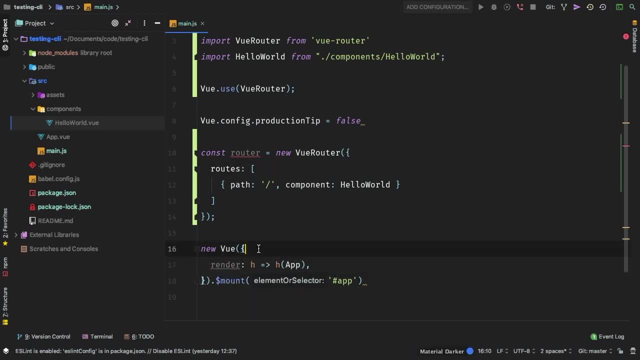 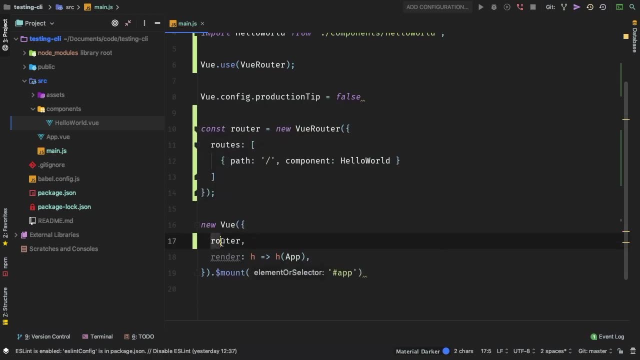 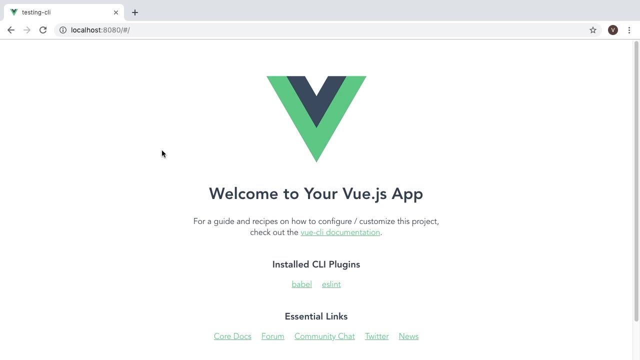 our routes, but we haven't told view about it just yet. So simple way to do this is simply just to pass in router into our view instance. So this router is belonging to this view router that we created up here. Okay, let's take a look at it in the browser, If I hit refresh. 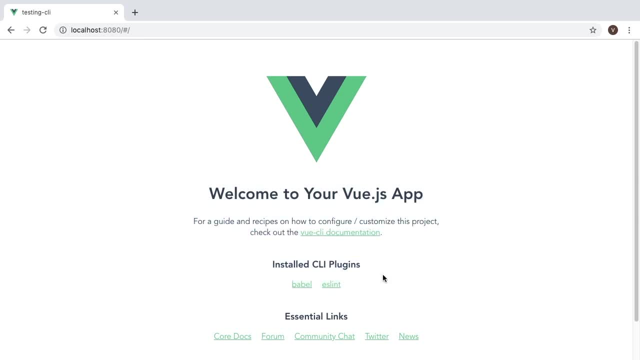 sure enough, nothing seems to have changed, But now we're actually routing. Now, one thing you'll notice right away is the following: is this right here? So there is a pound or hashtag, right here at the top, And this is due to the fact that browser support for single. 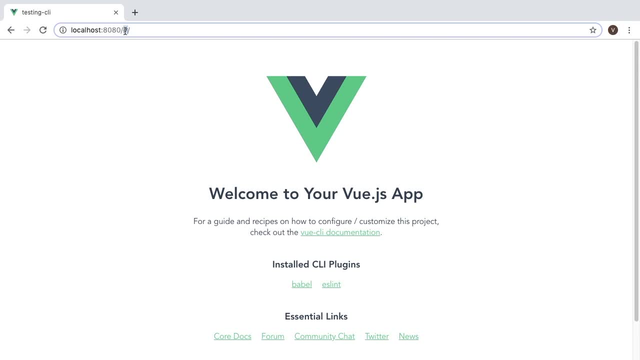 page applications isn't 100% yet. If you need to support older browsers like Internet Explorer, well, if you just route it between pages, it will actually refresh the page, which kills the whole point of a single page application. we don't want to ever have to reload this. 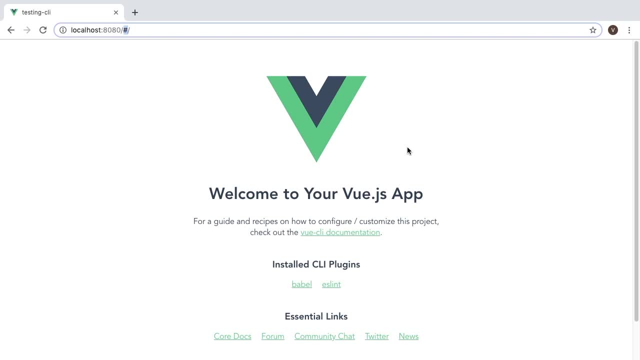 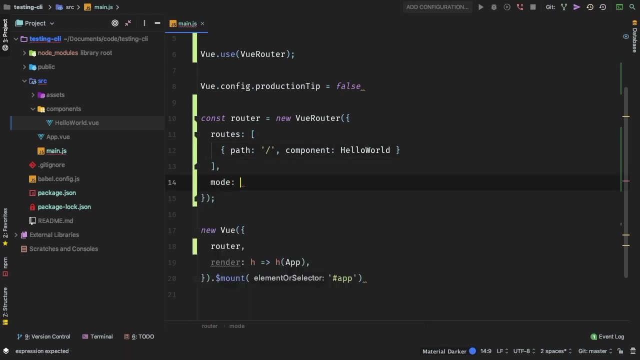 entire page, But rather we just want to load pieces or components of this page. Now, if you don't have to support older browsers, then we can turn this feature off, And that's actually very simple to do. Right after routes, we can add another one for mode And the mode. 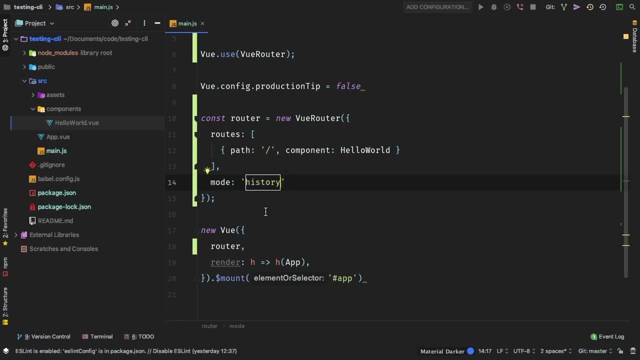 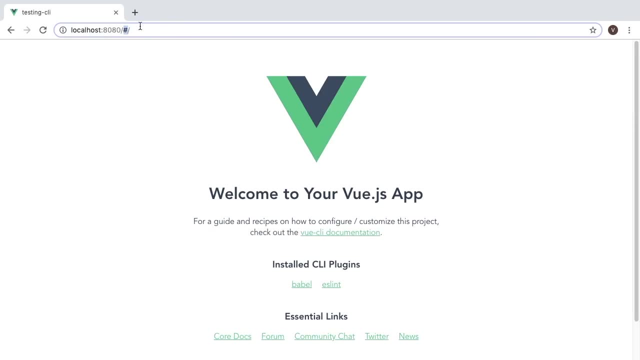 that we want is history mode. Now, history mode is going to use push state to push different content into the site And change the page. So we're going to go ahead and do that. So we're going to go ahead and change the address bar for us without needing that hash which looks a little bit ugly. So 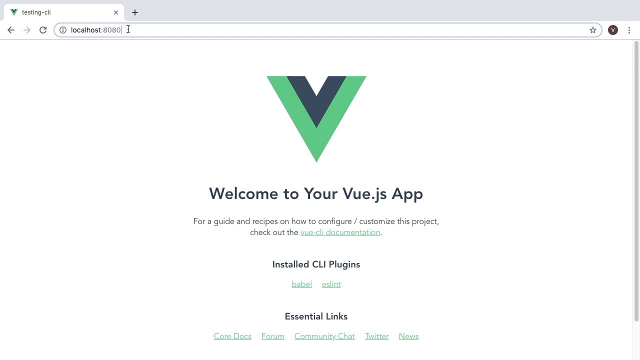 we can get rid of that. go ahead and hit that, And now we don't have that any longer. Again, if we turn this off and we go back to our page, it will automatically always add that pound. There it is, you see, it doesn't matter. I cannot get rid of it. But again, if we use 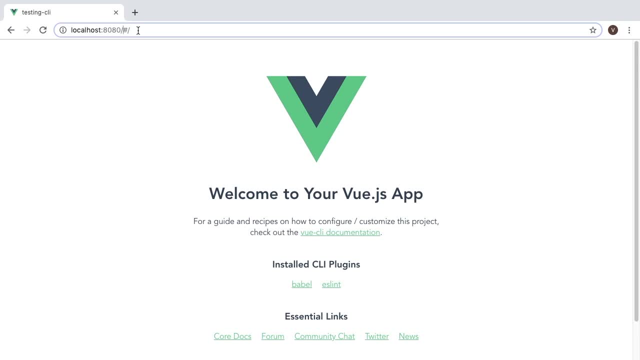 mode of history. in that case, then we can get rid of it all together And we just get a nicer URL Again. the point of that is just for older browser support of single page applications- Awesome. So why don't we create a new component? 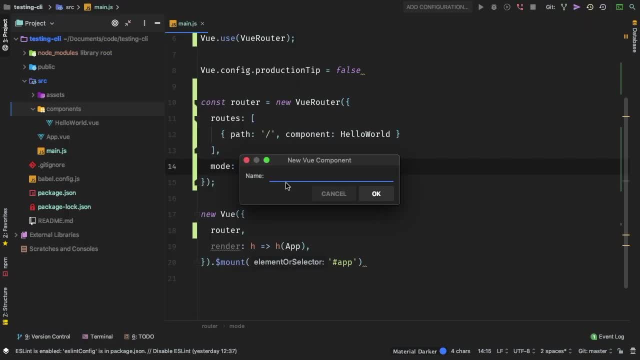 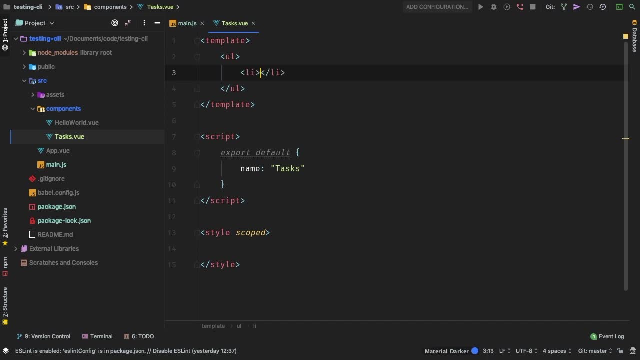 And then let's go ahead and create a new page. So let's add a new view component here And let's just maybe call it tasks, And inside my task controller I'm not going to have anything, but just some LI items. we'll just say item one, item two and item three. Okay, 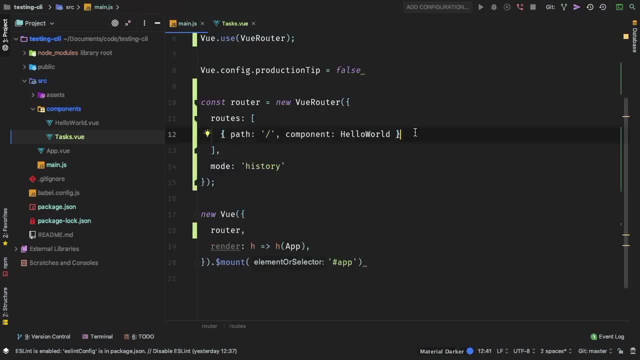 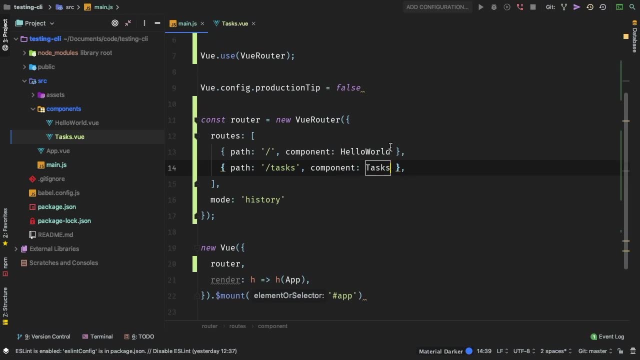 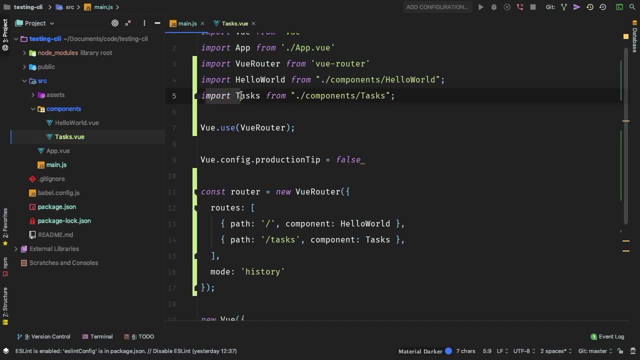 very simple component, nothing crazy. Okay, I'm going to actually copy this over And when I visit slash tasks, I want to load my tasks components Now up here at the top. it was imported for me automatically. again, just an ID feature. If you're not using an ID like me, go ahead. 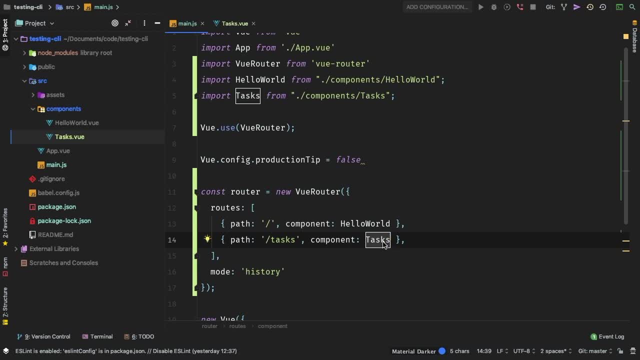 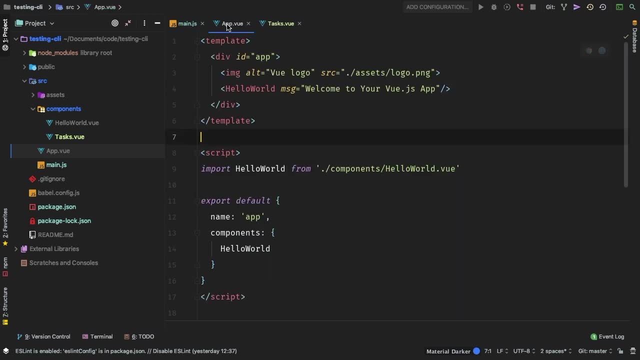 and add that line to the top, Otherwise your compiler is not going to be able to find tasks. So we're just about ready to test this. But if we did right now, it wouldn't work. So let's visit the app dot view, And right now we're loading Hello world. it's a component. 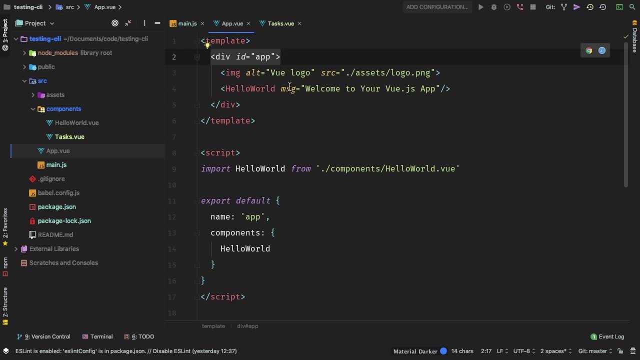 but we are already loading it inside our app, right inside our main view component. So let's get rid of this altogether, And what we need to put in here is router view. So router view is what's going to tell the router where to put your component. this is where you want. 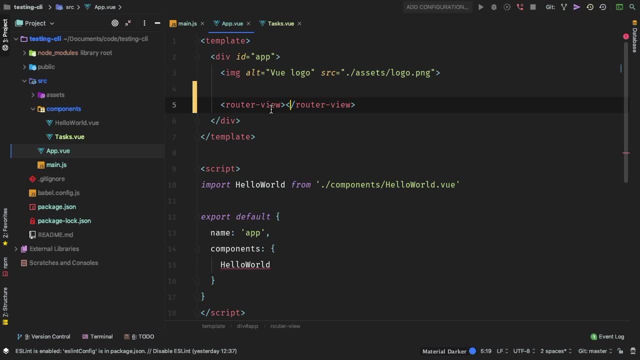 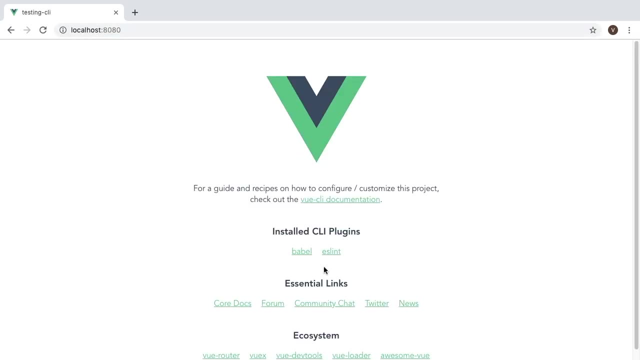 it to place your component. That's the point of router view. Alright, let's actually check it out in the browser Now. And there we go. we do see our list Now. if we head back into just our homepage, then we see that other component and the component we're loading. 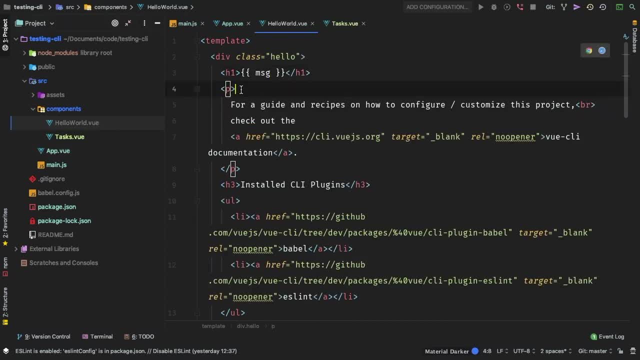 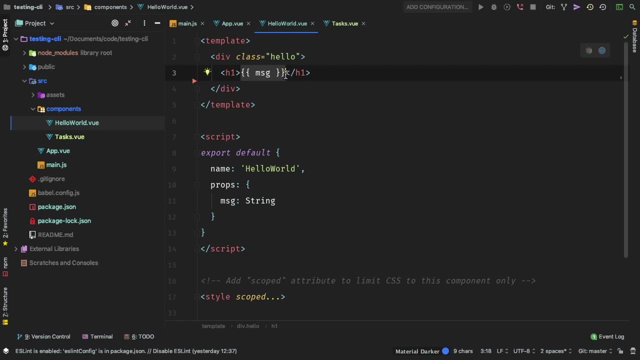 there is the Hello world component. Why don't we change this up a little bit, just so that we know that we are loading this component and go ahead and get rid of everything? And instead of a message, why don't we just output Hello world And there we go, So we have Hello. 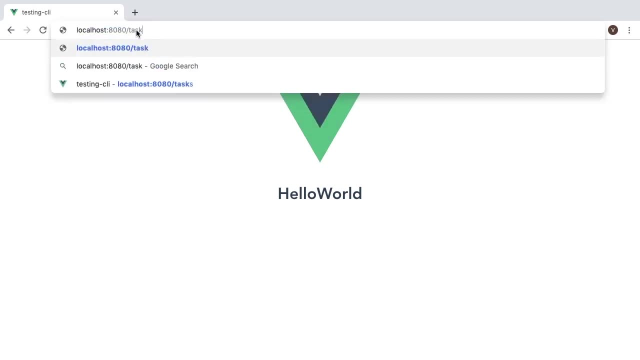 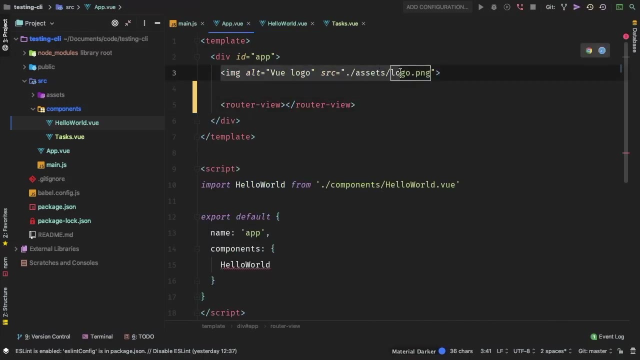 world component, And then if we visit slash tasks, then we have our tasks list. Now, this image up here, that's actually inside our app view And it is right here. we don't really need it, So why don't we get rid of it? 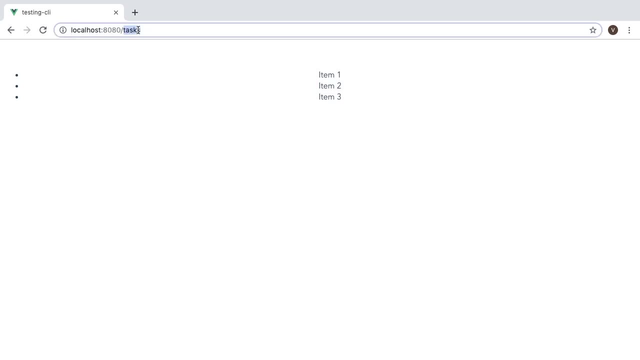 So now we're going to go ahead and load this component And we're going to go ahead and refresh this, then sure enough. and then if we go back to just slash, but right now the way that we're doing this, if you notice up here, right where the refresh is, you'll 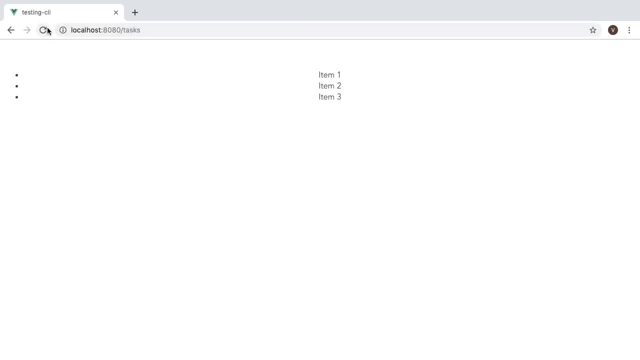 notice, when I go to slash tasks, it actually reloads the page. So right now it's still not a single page application, And the reason for that, of course, is that we need to actually generate some links that view can tap into. So why don't we create an imaginary navigation? 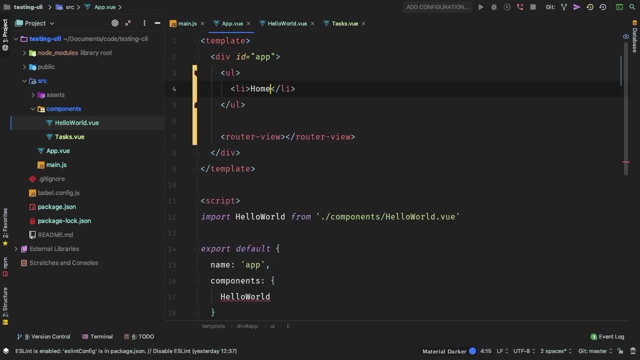 bar here with some unordered links By default. let's say, I've got some unordered list elements, So my first one might be home And my second one is going to be tasks. right, just something for us to be able to click through. So what we need to put in here is another view component element that gets added. 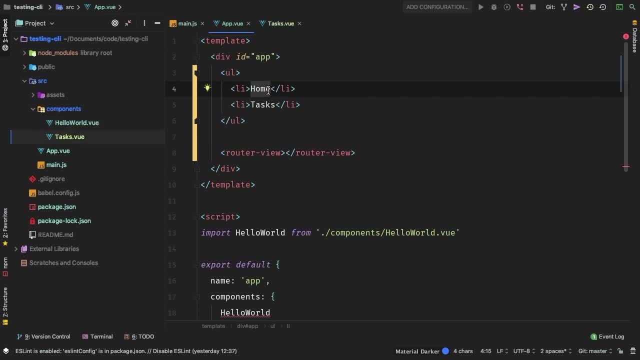 whenever you pull in view router and that is router link. So let's copy this out. Let's add a new component: router dash link And inside router link. that's what we're going to put home. So this is going to take one attribute and it's going to be the to attribute. 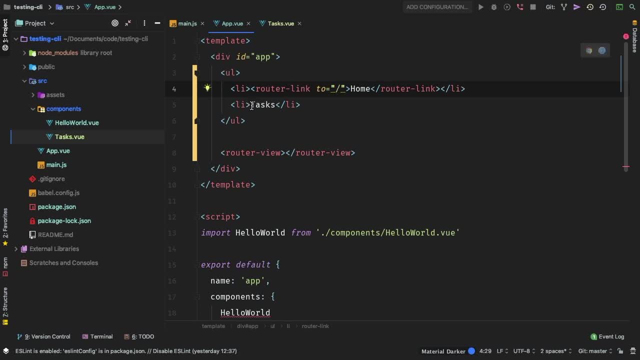 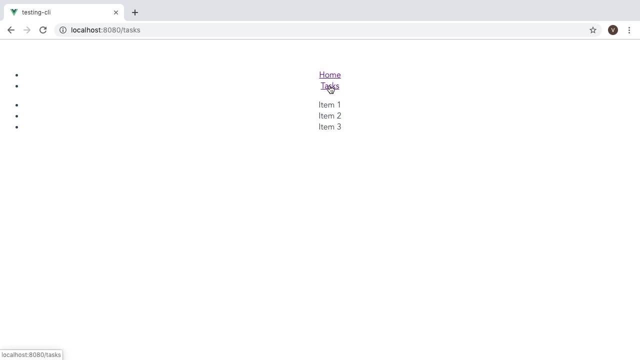 So where are we going here? we're just going to slash Similarly for tasks. let me go ahead and grab that And let's add a new router link. paste that back in and this is going to go to slash tasks. Okay, so back in our application. now these have turned into links. 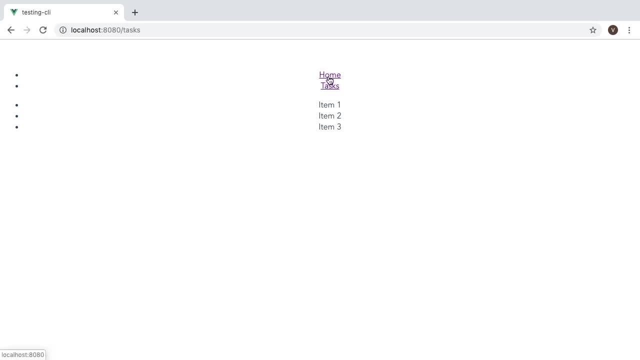 Now pay attention up here, right where the refresh button is. let's go to home and tasks. Notice how there's zero loading between these two. we're not refreshing the page. So we have successfully actually added some routes and we are actually in a single page application. 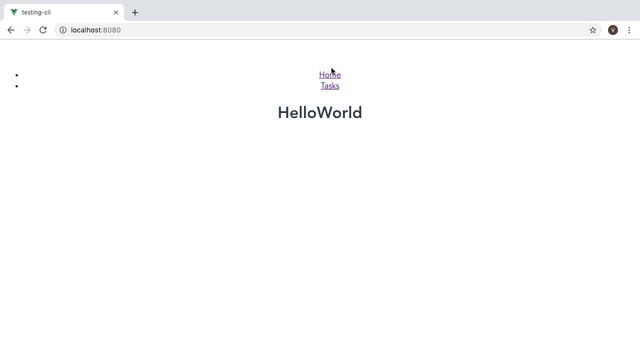 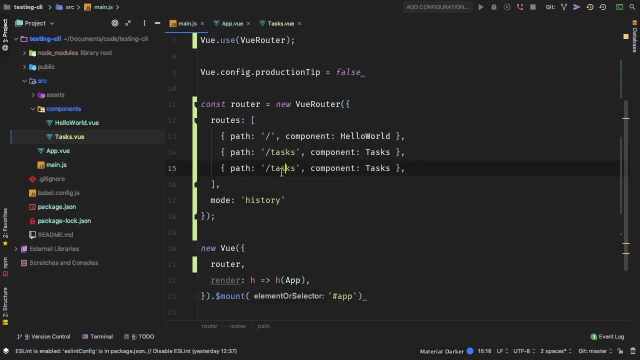 This is the very basics of view router and how to get everything working. But let's take it a step further. What if we wanted to pass some parameters? Let's say the following: let's add a new route here, And this is a common thing. let's say user, and then we're. 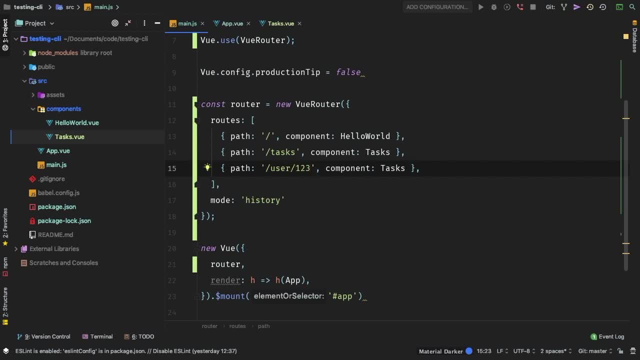 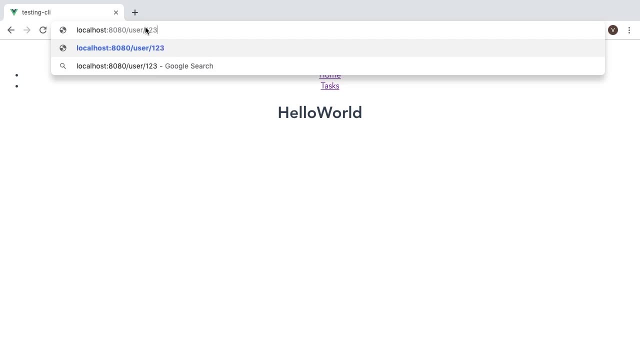 going to need an ID of a user, say ID 123. Now we don't want to hard code 123. Because obviously every user is going to have their own ID. So sure, 123 would work, But 1234, that doesn't work. So this needs to be dynamic, So very. 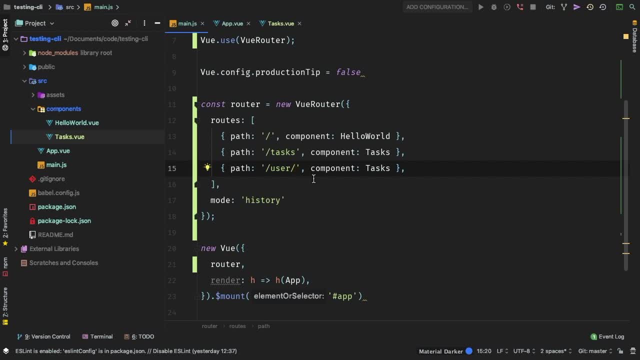 similar to how view assigns something and binds it. we can actually use the same notation of semi colon and then maybe we can call it ID. you can also call it user underscore ID, whatever you'd like. we'll just stick to ID for now. So now view knows that this. 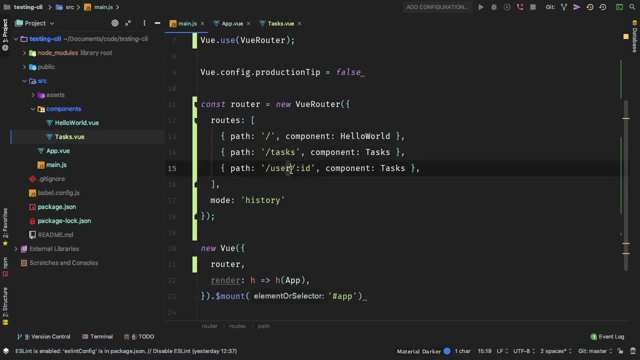 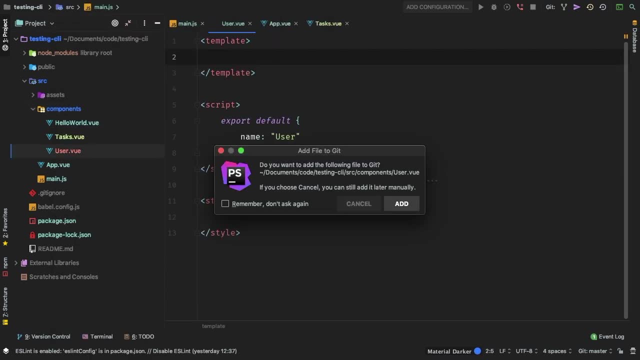 is actually a variable and not just a regular string. So why don't we create a new component And let's go back here and add a new view component for my user? So this is a new component And all we're going to do here is just very simple. Obviously, we're just trying to get 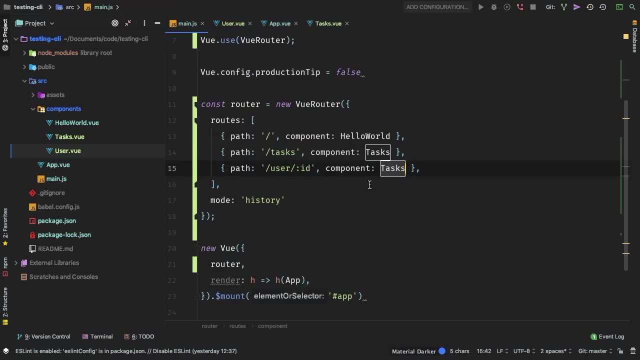 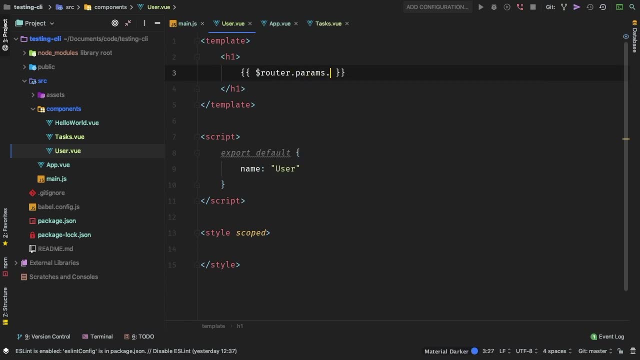 this working, So we're going to go ahead and output out. So how do we get access to this variable right here? Well, very simple. You're going to reach for router, dot, params, dot ID. Again, router is just a global instance of router, the same one that we gave in here and then. 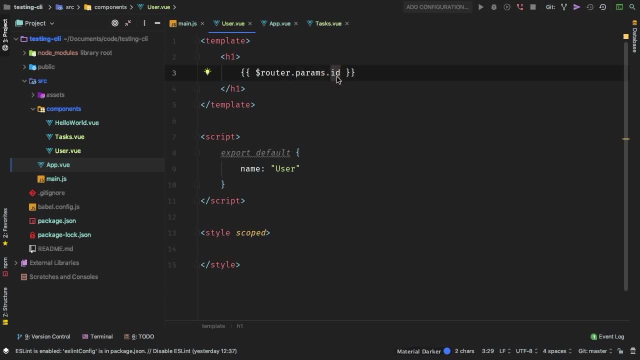 params, meaning any available variables, and then ID, which is what's belonging to our ID right here. If I change this to user, then of course I'd have to change this to user instead. That's the connection there, So we'll keep it at ID. I'll put everything back to. 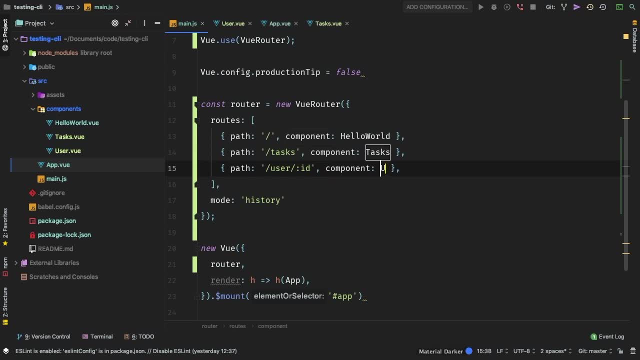 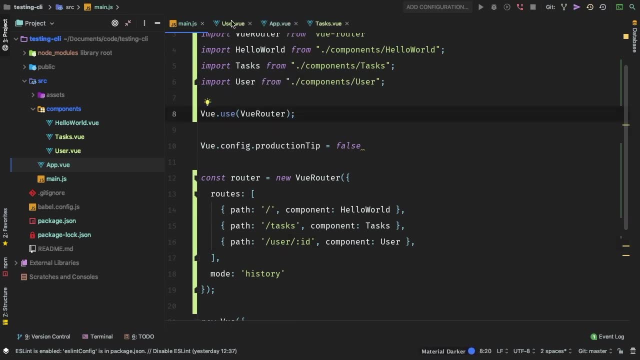 ID. And now, instead of tasks, then of course, we're going to use our new user component. This user component did get imported up here at the top, So let's go ahead and try this now in our browser. Before we do, let's go ahead and add this new route to our route links. So, user slash. 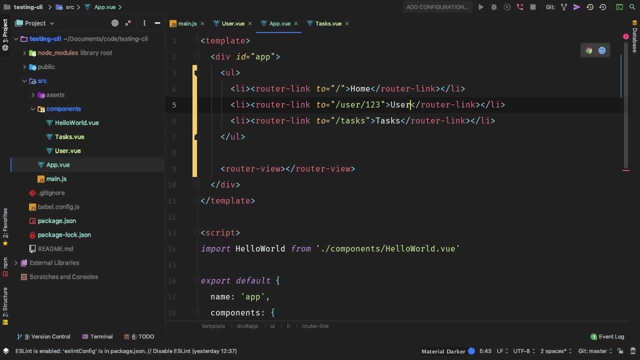 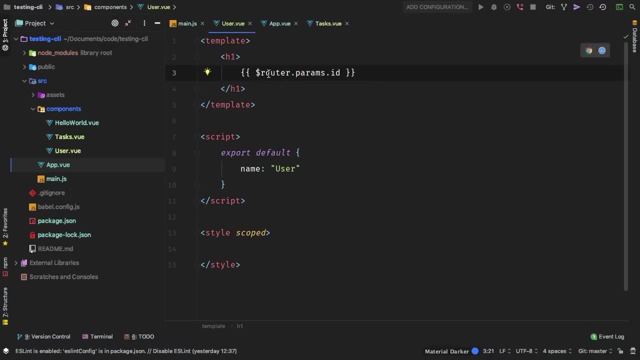 we'll just say 123 for now And then just call it user. All right, let's head back here. Let's see user. All right, that didn't work. Let's go back here and check what happened. Okay, it's not router, it's route. So, reaching out for route params ID And there we go. 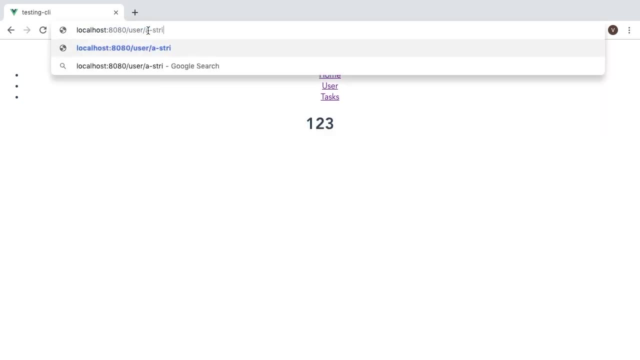 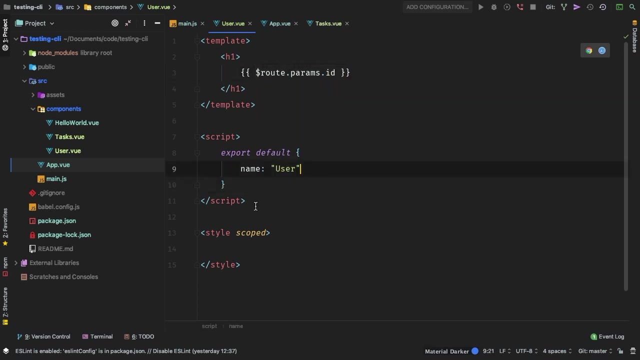 Now we're getting 123.. So anything we passed in in here, the string also works through 1234.. Yep, that all works. So we are successfully fetching that. not obviously in the real world At this point. you would maybe fetch that user's information and show their profile. 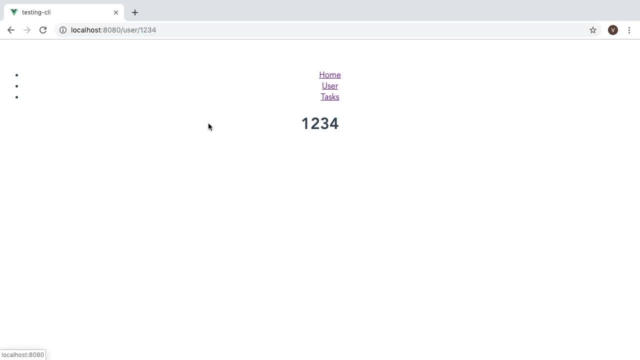 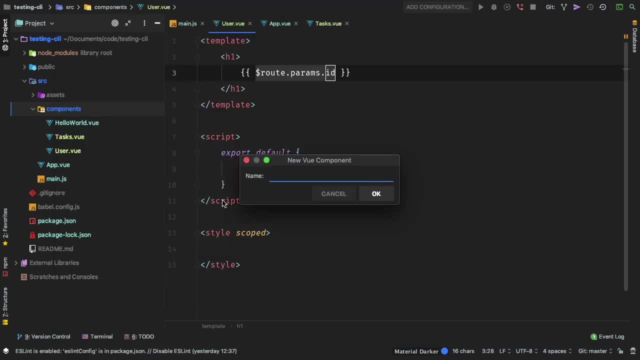 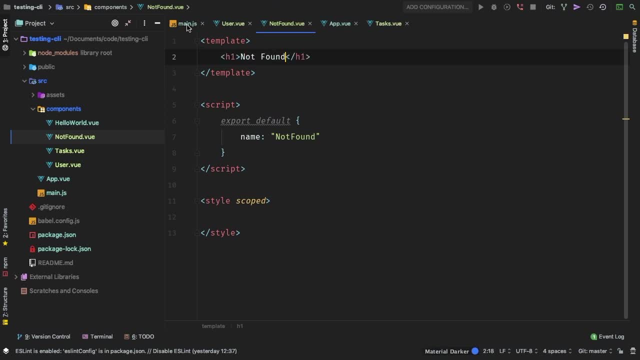 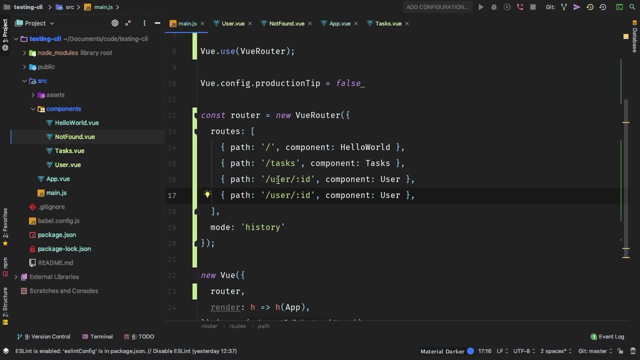 going to be just an h1 that says not found. So now my main dot. just let's add a new route. Now we want to catch everything right, Everything that trickles down. think of your route as the users appear and it's falling through these different routes. So the first match. 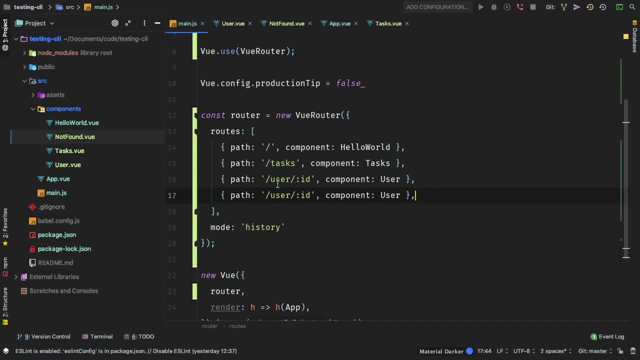 that occurs will be the one that actually gets returned. So at the very end, this very last, what we can do here is put an asterisk And this will basically just tell view router anything else. if it all fails and it ends up over here, go ahead and match everything, And if it matches, 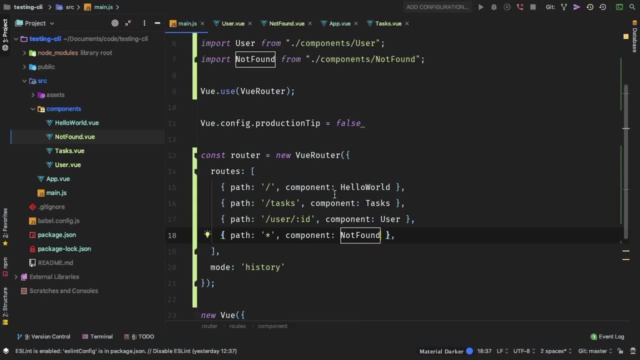 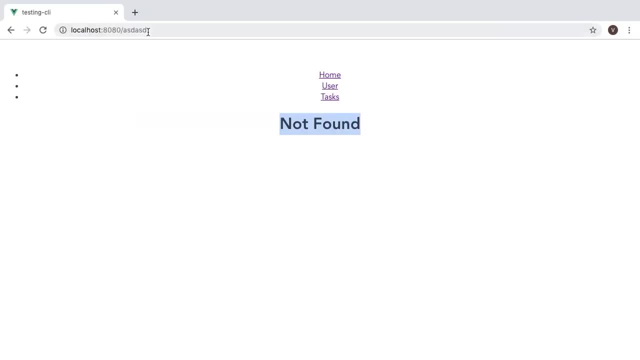 everything. let's go ahead and pull open the not found component. not found, that imported up here at the top. So keep that in mind. So now when we come back here, sure enough, we get not found, But all of our other routes still work. Now the order of these routes is very important. 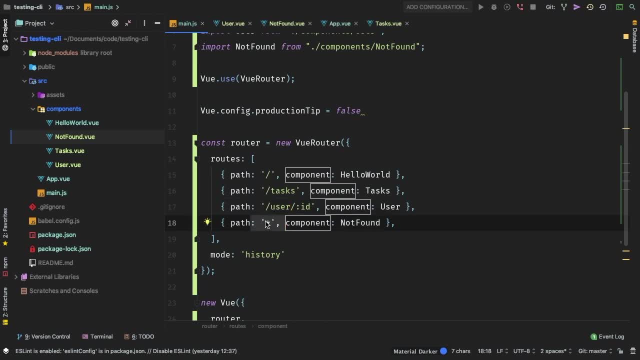 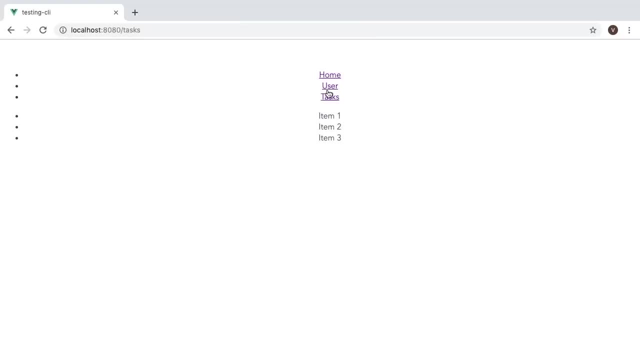 you want it to have that trickle effect. So at the end is where you're going to have your wildcards. That way you don't accidentally overwrite one of your other routes. So that's pretty cool. This is pretty easy to implement And, again, 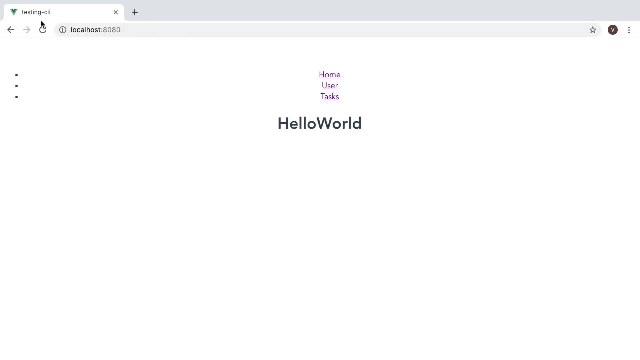 we have all of this working without refreshing the page not even once Now. we still do have history, So if we click through here, you see that we still have history going on up here, But again, we're not reloading the page. So everything is extremely fast and easy for the user.